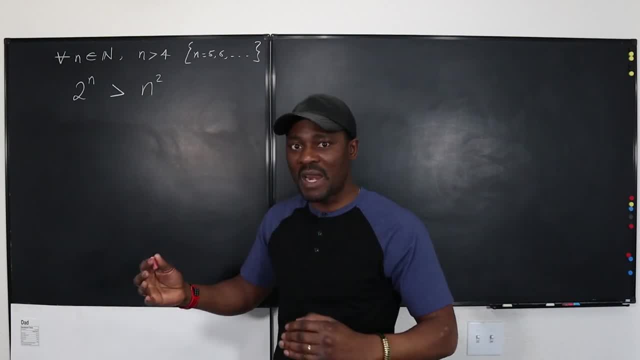 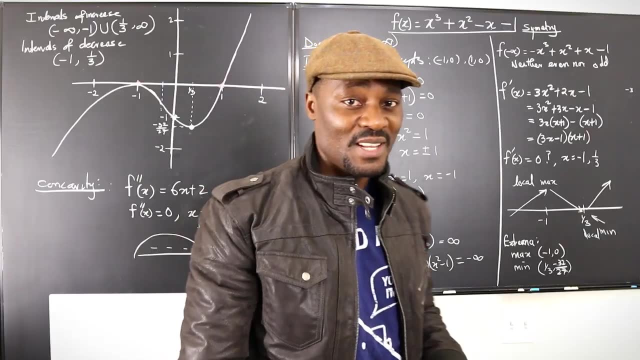 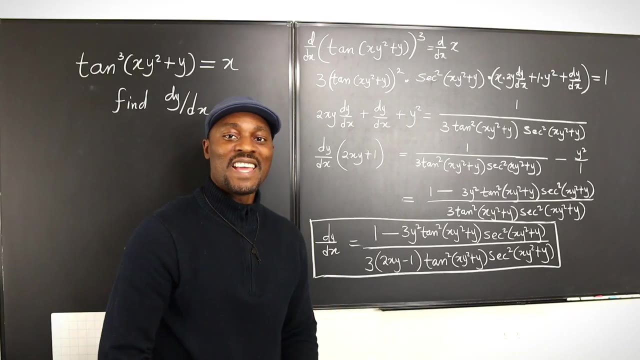 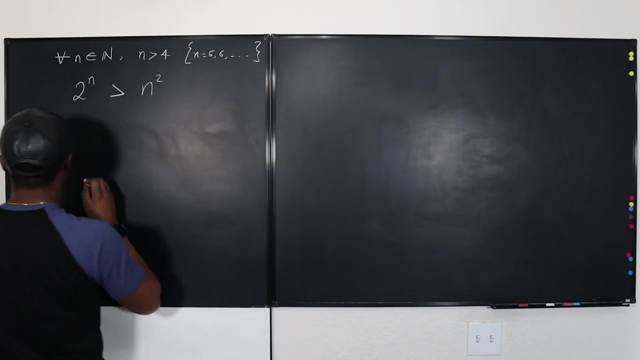 follow the three other steps and do your manipulation. You get your answer. Let's get into it. The first thing we're going to say is that our proposition is for n, such that 2 to the n is greater than n squared. Remember, this question says n has to be greater than 4.. 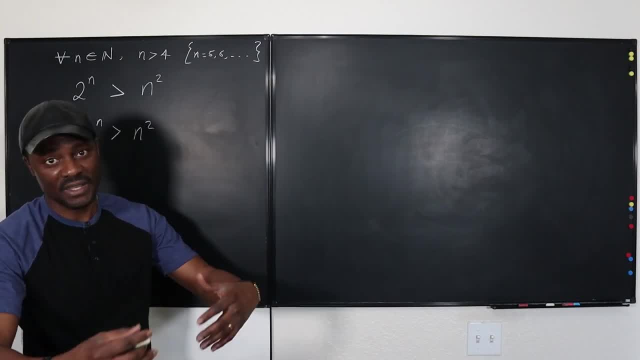 So the first natural number after 4 has to be 5,, 6,, 7.. So those are the numbers we're working with. So the second thing we're going to say is that our proposition is for n, such that 2 to the n is greater than 5.. So the second proposition is to start. we're going to test. 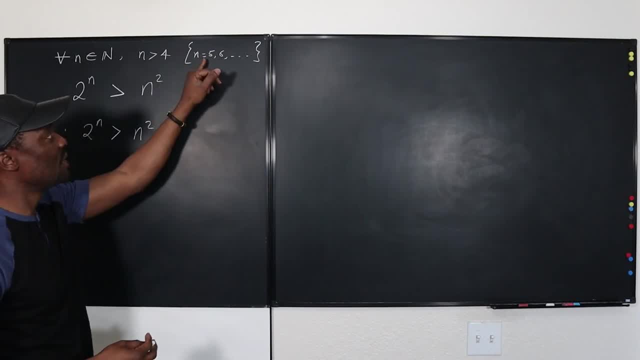 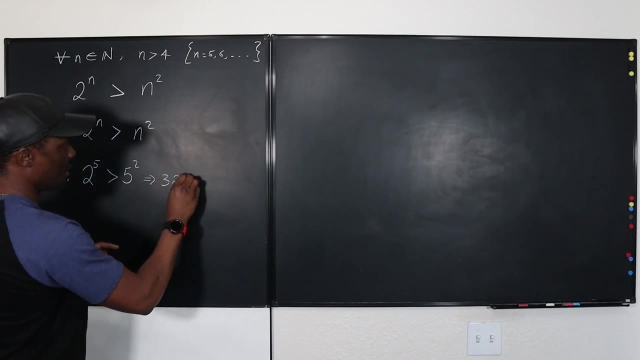 So the second step is to test the first available number, which is 5.. So we're going to test the proposition for when n is equal to 5.. Okay, so we're going to show that 2 raised to the power of 5 is greater than 5 squared. Okay, is this true? Which implies 32 is greater. 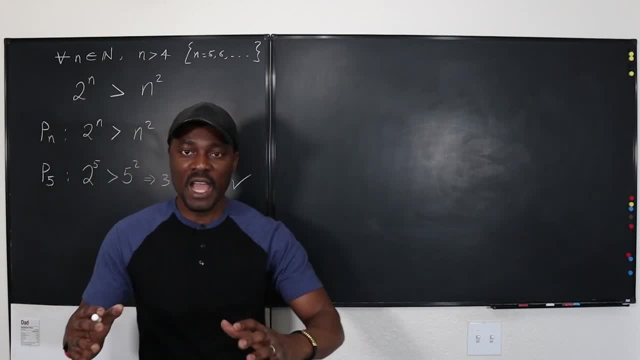 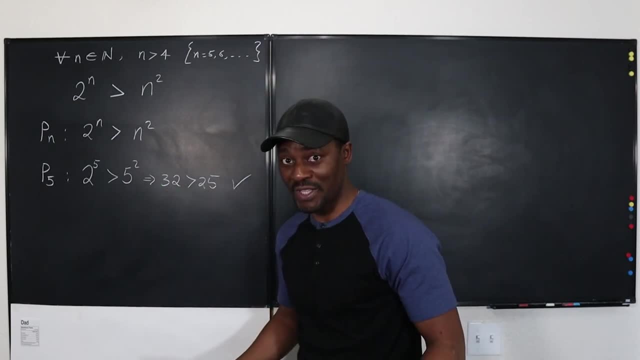 than 25.. Well, this is a true statement. So now, because we're starting from, n equals 5,, 6,, 7, this statement is true, So we go to step 3.. Step 3 is to make an assumption that if we pick any of these numbers in the 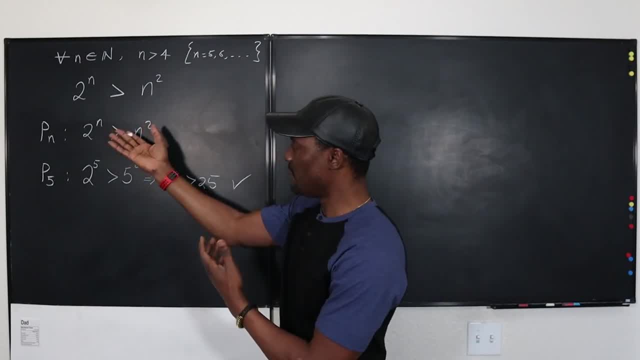 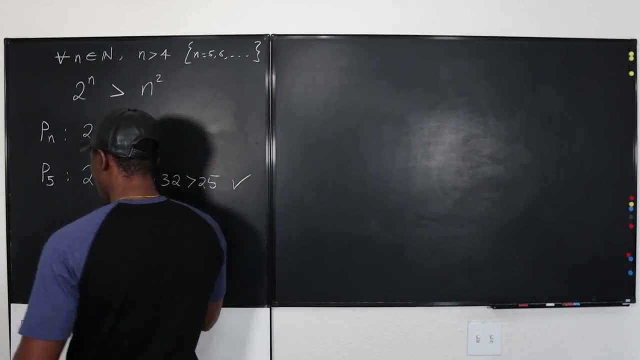 future we're going to get a true statement. That is, if you pick 5 or 6 or 7 or any number, so we're just going to take any number k And we're going to say: the third step is the. 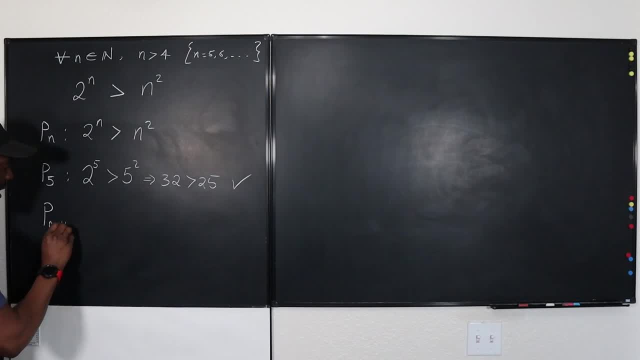 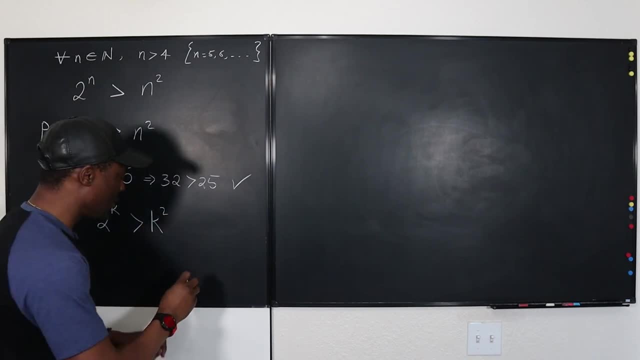 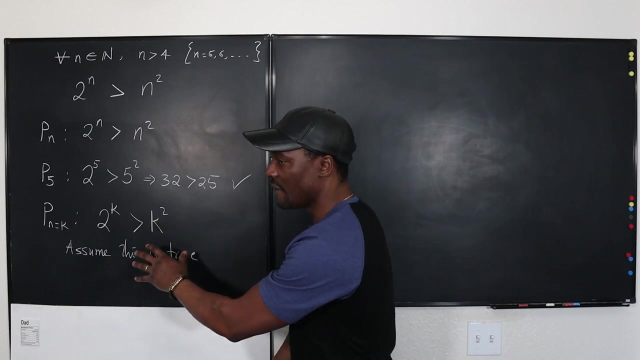 proposition where n is equal to k, okay, is such that 2 to the k is greater than k squared. Now this we have to assume. assume this is true. So this is the bedrock of all mathematical induction proofs, This statement that certain k in the future or anywhere, starting from. 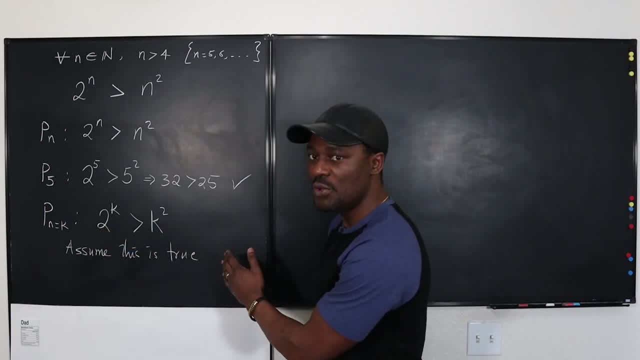 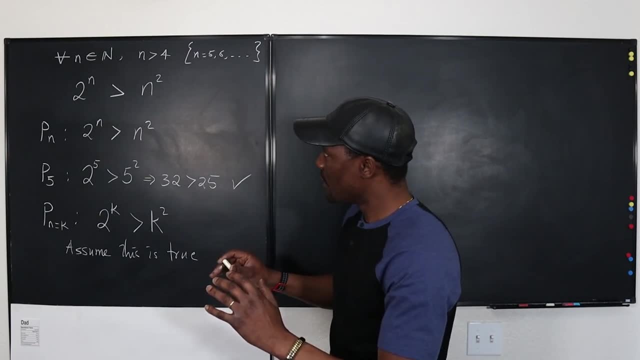 5 will be true is what you then use in the next line, which is the fourth part of what we're doing Now. The question is: why didn't we start from 1? Will it always be true? Why can't since? 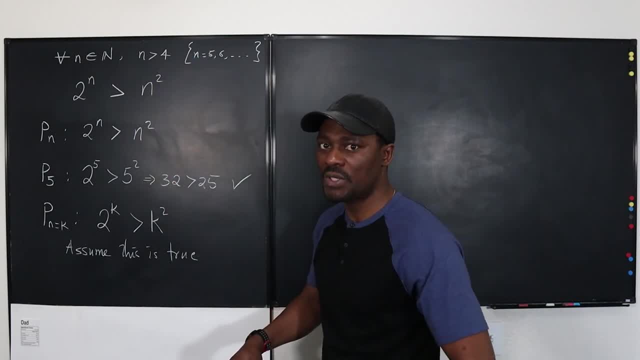 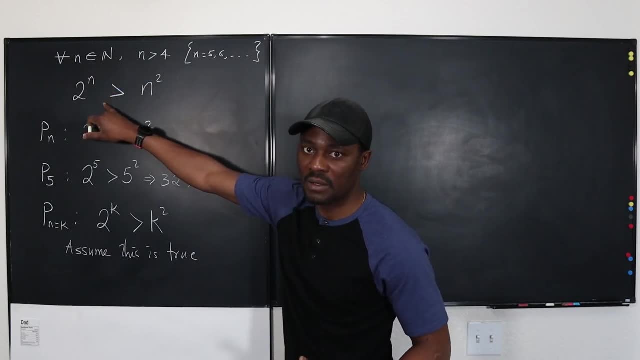 we already tested 5, why can't we just say to be true for 6, true for 7, true for 8, and so on, since it's already true for 5?? The problem is, it was true for 1,. okay If. 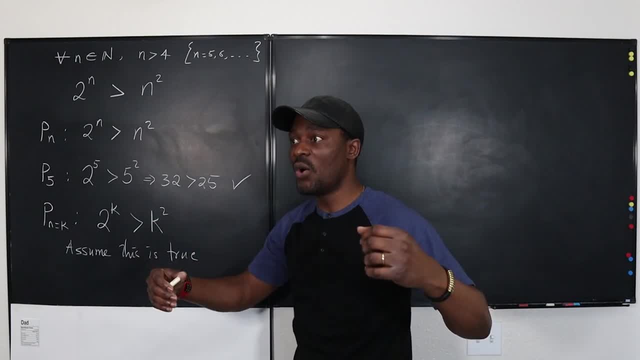 we don't test every number, you would end up saying, oh, it is always true or not always true. Look at this: If we test it for 2 raised to the power of 1, it's going to be 2 is greater. 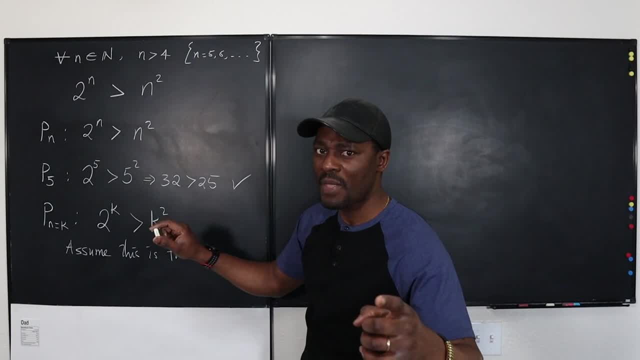 than 1 squared, 2 is greater than 1.. That's true, But it's not true for 2, because 2 squared is not greater than 2 squared. You see, they're not, it's not greater. It's not true for 3, because 2 raised to the power of 3 is 8.. 8. 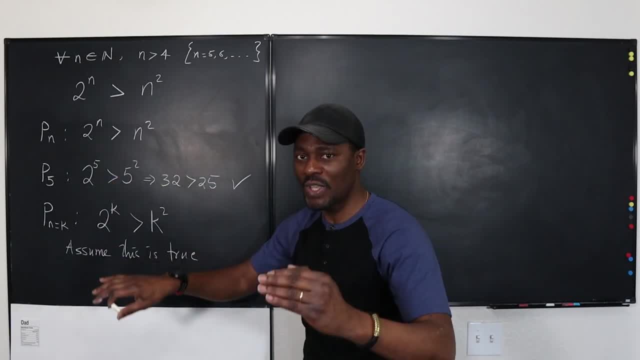 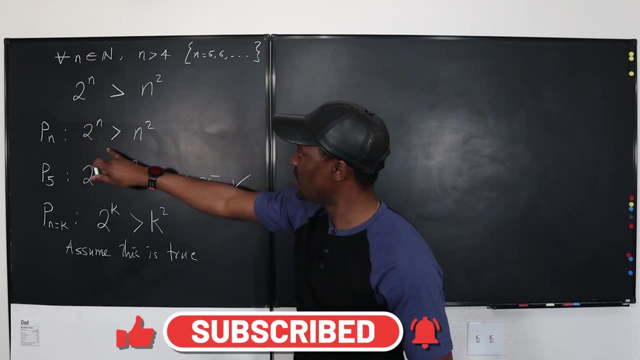 is not greater than 3 squared, which is 9.. So that's not true. So you can see: true, not true, not true. And if you test 4,, 4 is going to be 2 to the fourth, So it's 16 is greater. 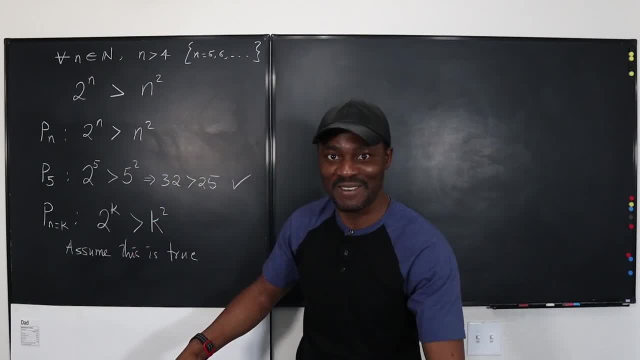 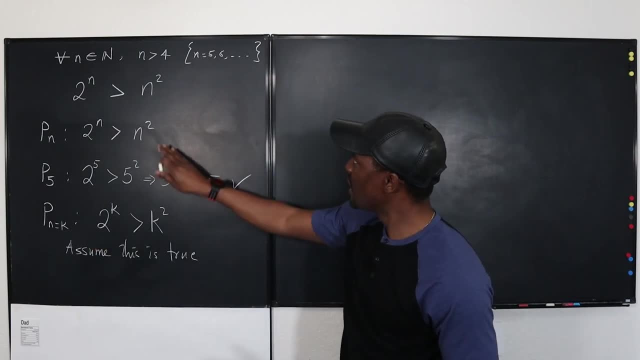 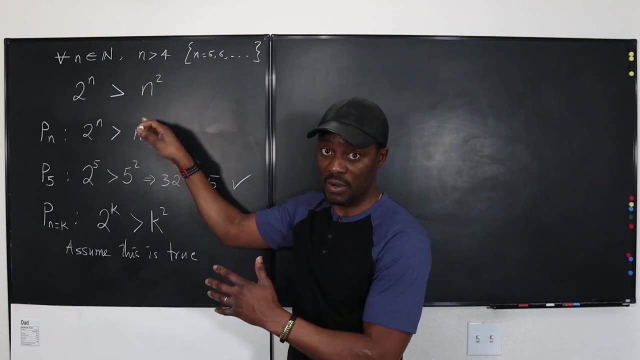 than 16.. That also is not true, But when you get to 5, it's true again. Okay, So the point of this is, you want to make sure that this assumption you've made is within the numbers that we are working on. We're already confirmed: it's not true for up to 4.. It's only true. 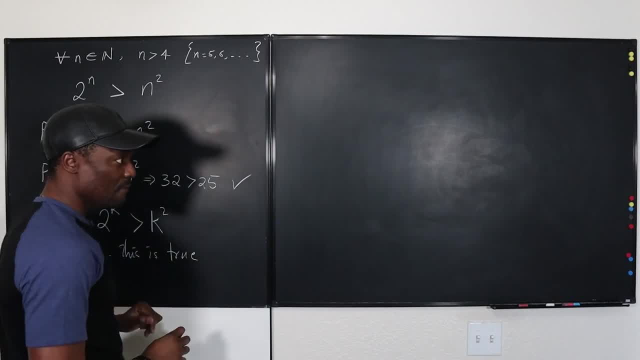 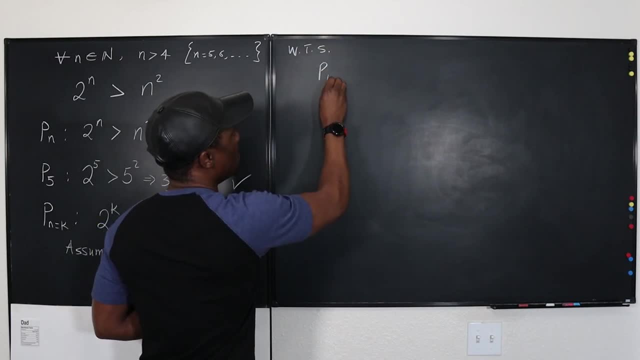 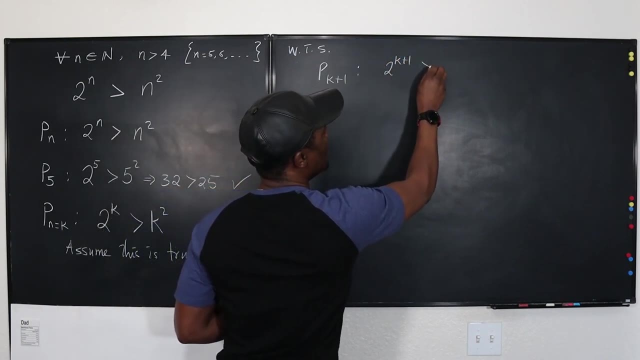 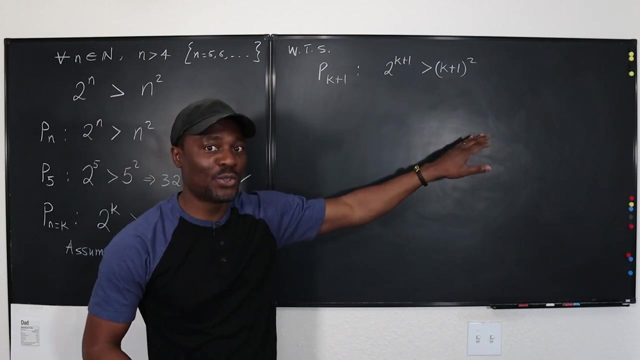 for the beginning, 1.. So now, what do you do? The next thing we want to prove, we want to show that the proposition for n equals k plus 1, such that 2 to the k plus 1 is greater than k plus 1 squared. Okay, So this is what we want to show: that this is true. But we 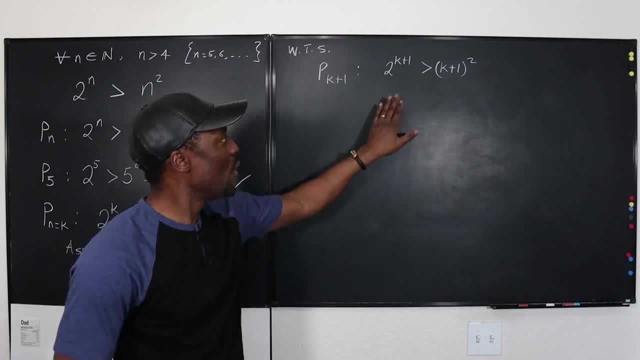 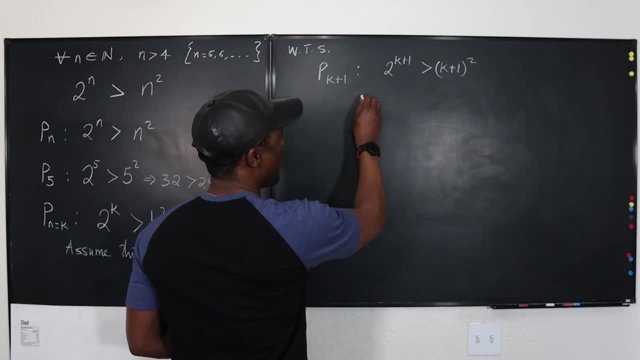 don't know if this is always true. So what we're going to do is work with the left-hand side and see if we can arrive at the right-hand side. So let's just do our basic algebra here. So what we have is: this is the same thing as. so let's do the work here. So we have. 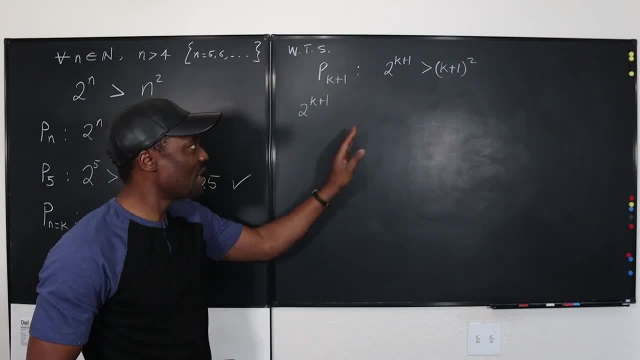 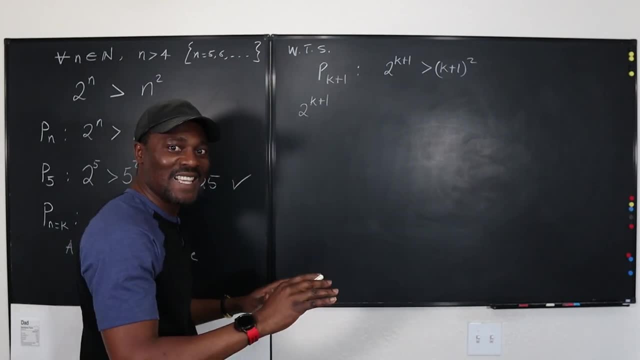 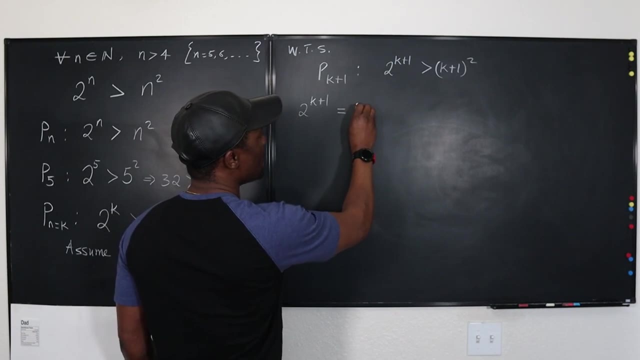 2 to the k plus 1.. Now see, I want to get this at the end, Okay. So in this case, I might just continue on a straight line, which is very straightforward, Or I might go this way. I choose my method. Okay, This is the same thing as 2 to the k. 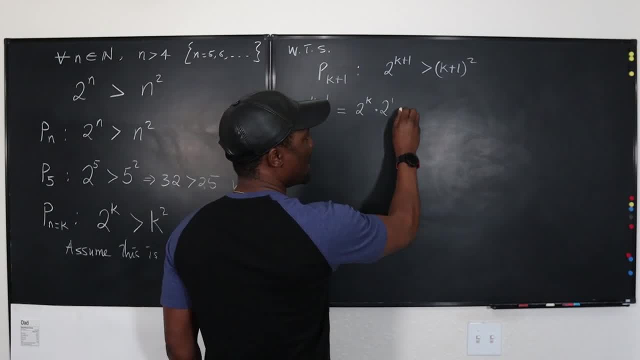 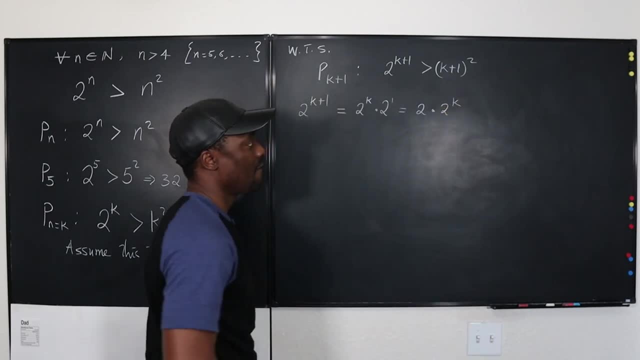 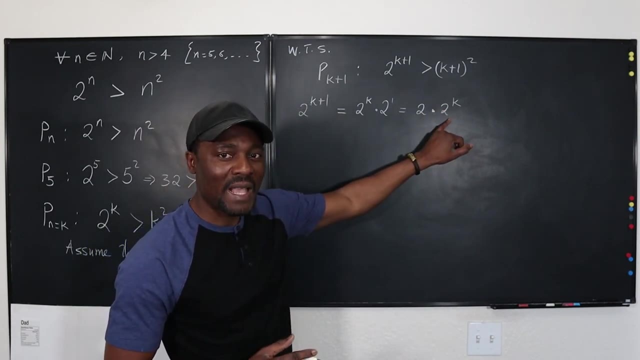 times 2 to the 1.. Okay, Which we can write as 2 times 2 to the k. So this is 2 times 2 to the k. Okay, Now I have to go back because I can work with 2 to the k. So you go back here and say 2. 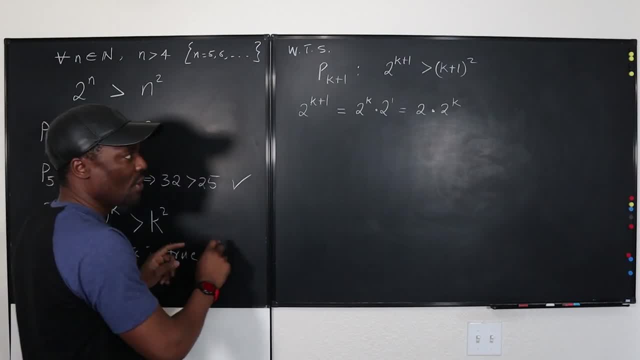 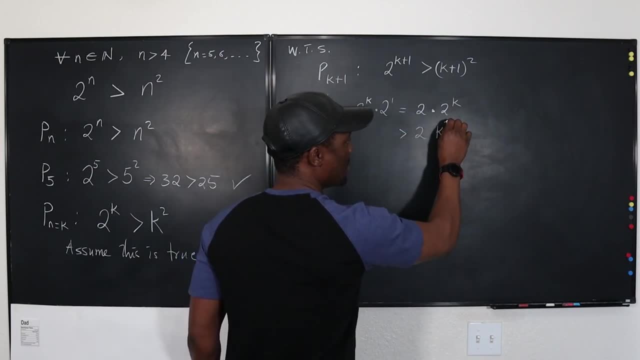 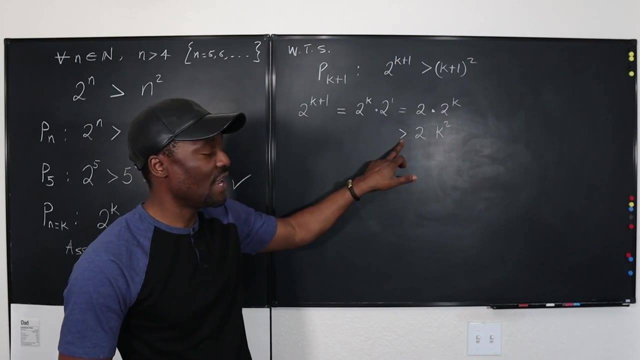 to the k is greater than k squared. So if I replace 2 to the k, I can say that this is greater than 2 times k squared, Because definitely k squared is not as big as 2 to the k. So I have immediately introduced an inequality. My mission is to transform this. 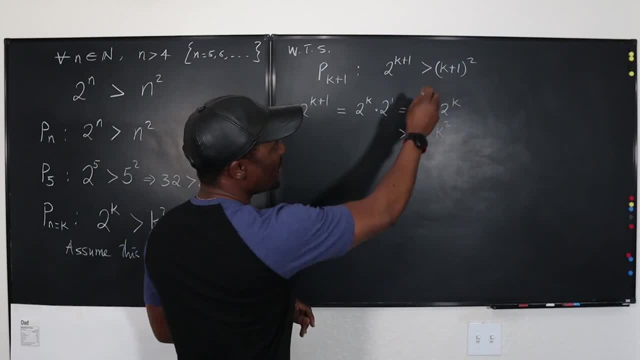 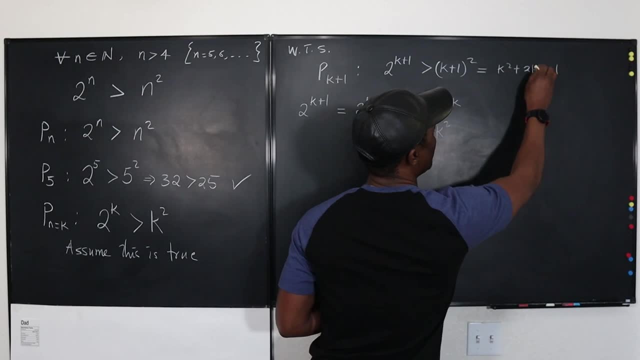 to look like this, Because I know that if I write this out, look at this. This expression is k squared plus 2k plus 1.. Do you see that? k squared plus 2k plus 1.. So this 2k squared, I only. 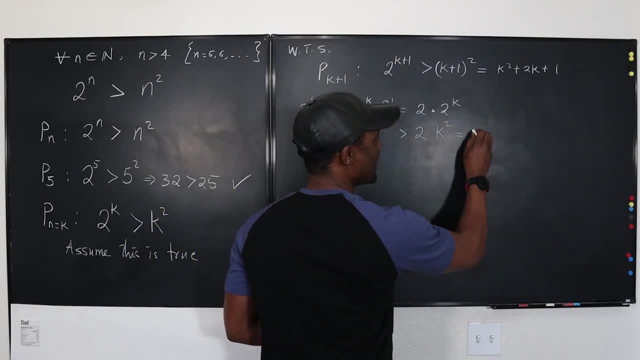 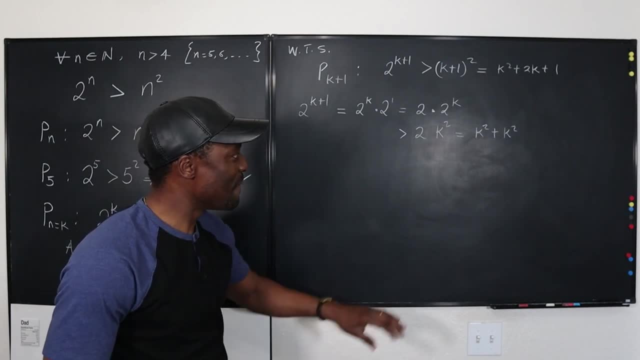 need 1k squared, So I'm going to rewrite this as k squared plus k squared. Nice, Okay, So I have k squared plus k squared. What can I do with this k squared? Because I need 2k. I don't need k squared. 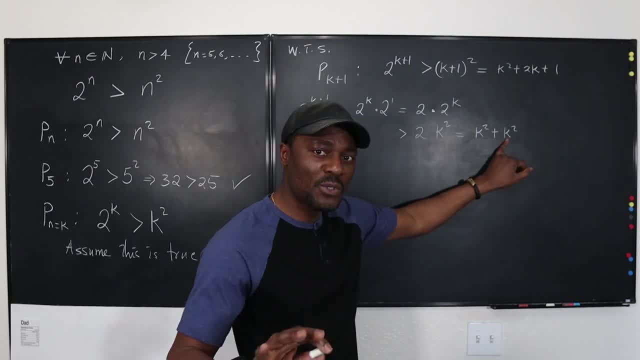 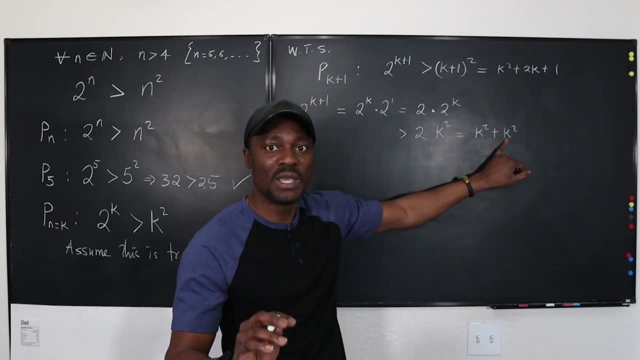 So remember that for all the numbers we're dealing with, we're dealing with 5,, 6,, 7.. So if I write k squared, the smallest k squared has to be 5 times 5, right, Which is 5k where. 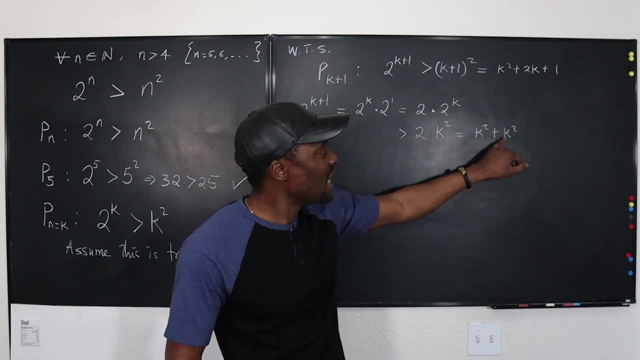 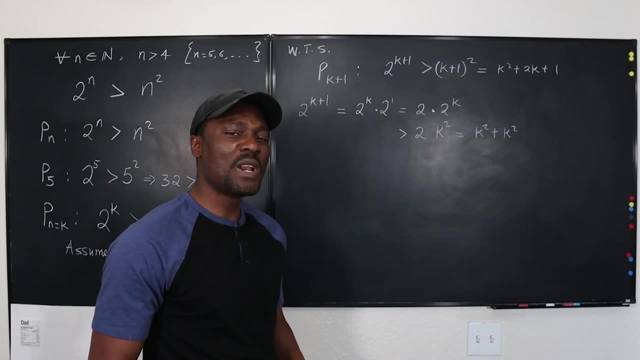 k has to be 5.. That's the smallest k, which is 25.. But what if I say I want to do 4k, This is equal. But that would be equal, But I don't want it to be equal, I want it to. 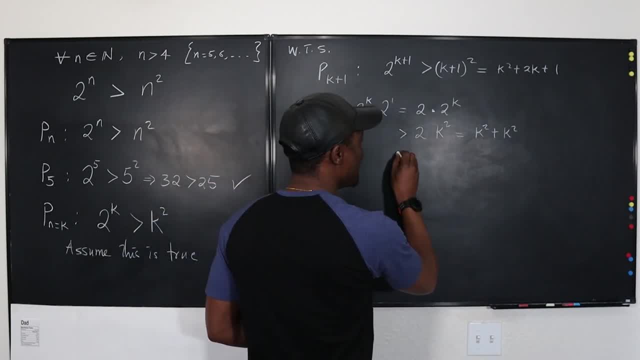 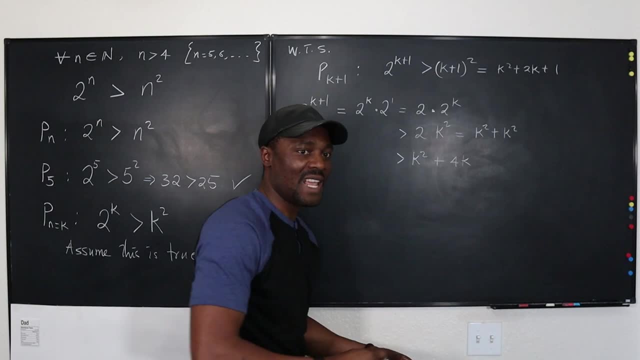 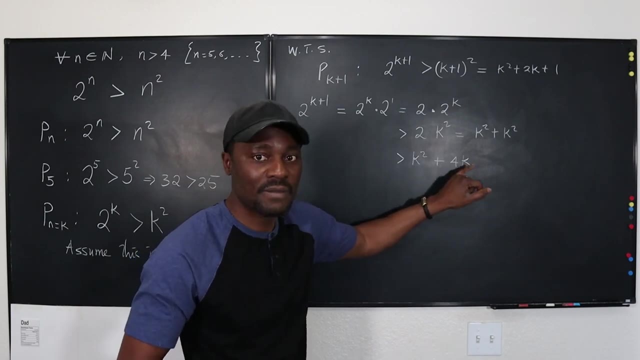 be greater. Okay, So I'm going to say this is greater than Now. see what happens. I'm going to write k squared plus 4k. What I've done is I have reduced the value of this, because this cannot. this shouldn't be 4k. The smallest we should have should be 5k, where k is another 5 or 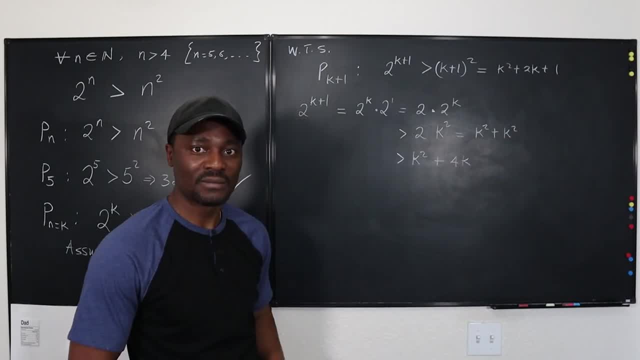 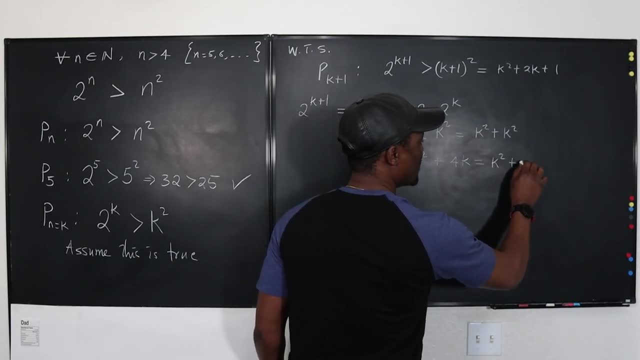 6 or 7.. So now I have 4k. I've changed this. Now I don't need 4k, I need 2k. So what I'm going to do is I'm going to write this as k squared plus 2k plus 2k.